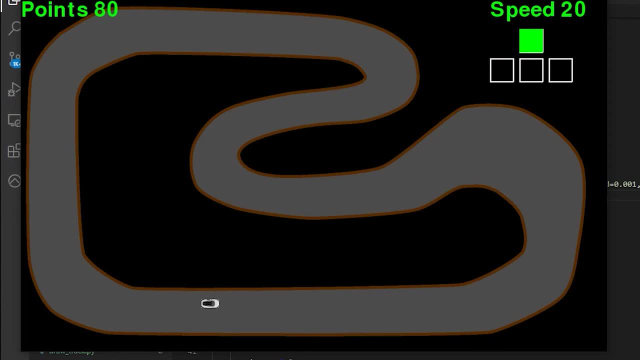 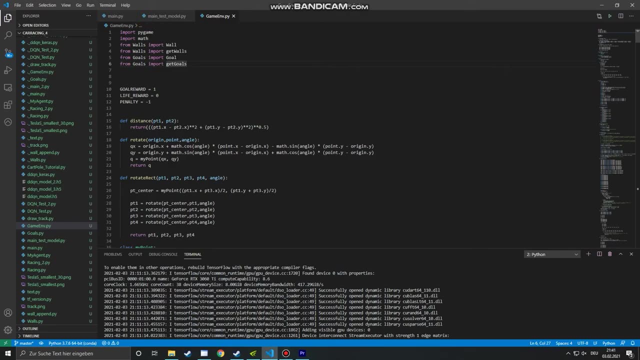 more about coding in Python and more about deep queue learning. So now I want to give you a short overview of how it's working. So the first thing I needed was a gaming environment which not only renders the game but also calculates the movement and calculates if there is a collision and keep track of the score. 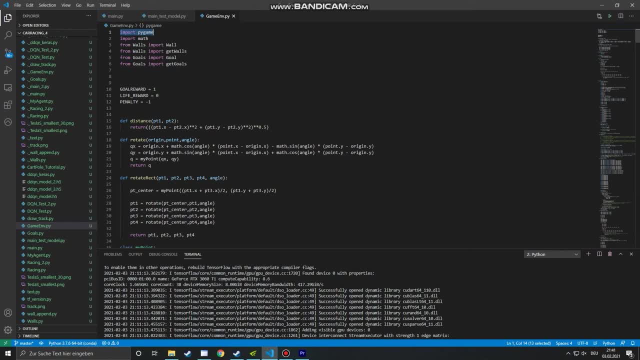 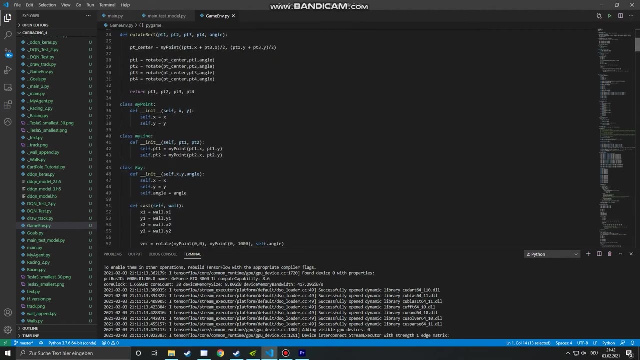 So I'm using Pygame for the basic rendering and stuff And this is a quite popular library to program games in Python. So there are a lot of classes and objects in the gaming environment, But the main ones are the car, the ray. 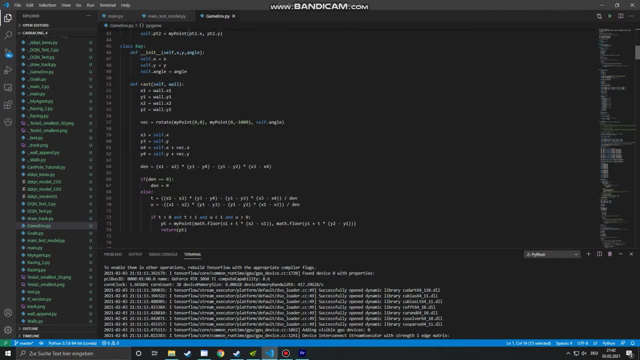 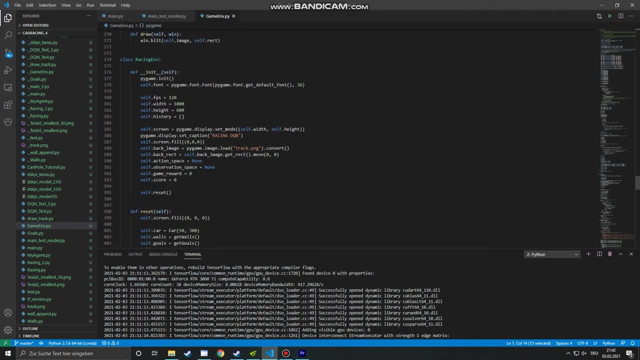 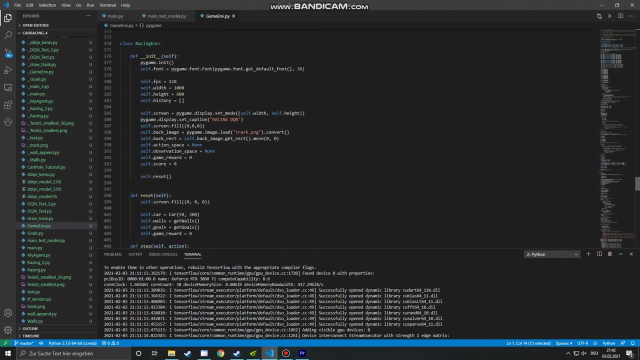 I will explain later how. for what we need the rays and the main game environment. Let's see Here it is. And the gaming environment has a defined set of functions which I will call, using my machine learning algorithm. So the first thing is we have an initiate function, as normal. 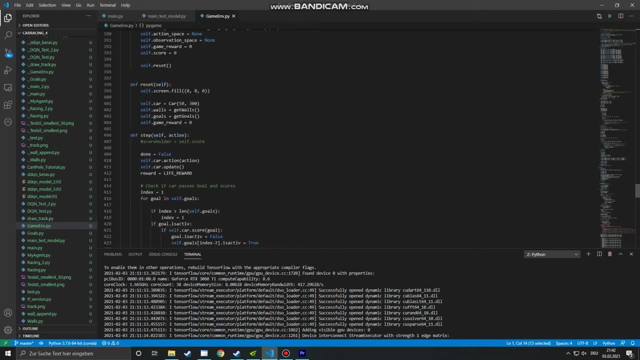 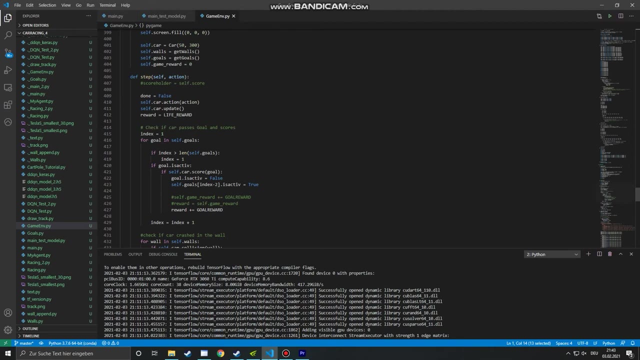 We have a reset. So if, for example, the car crashes into the wall, I want to reset. Then we have the step function. So we want to hand over a certain action and we want to to the car to respond accordingly. so, for example, if we move forward, then the car should move. 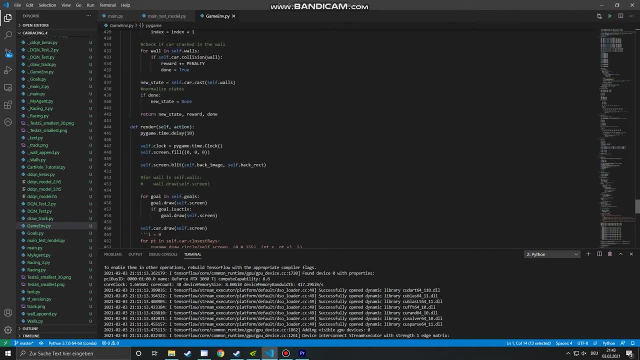 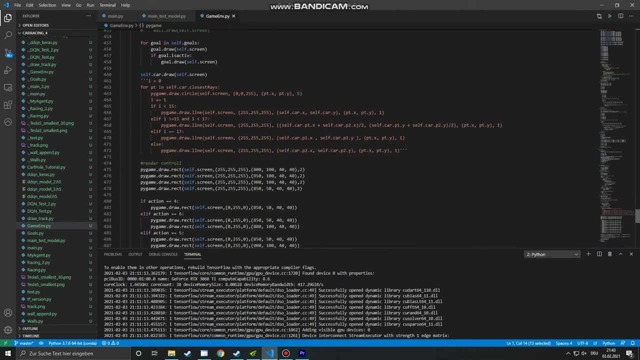 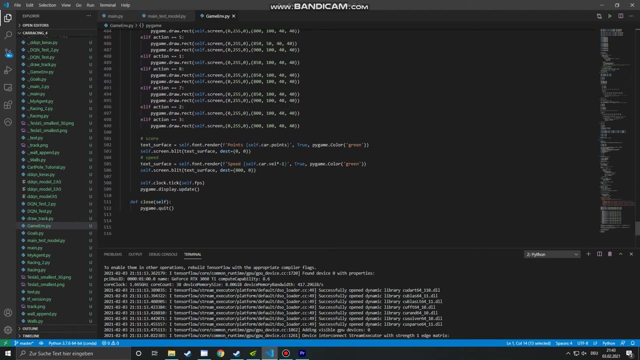 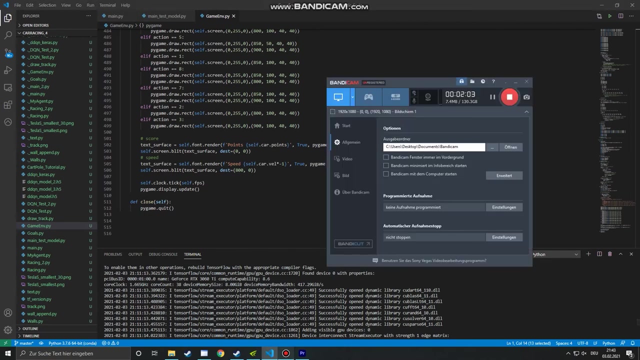 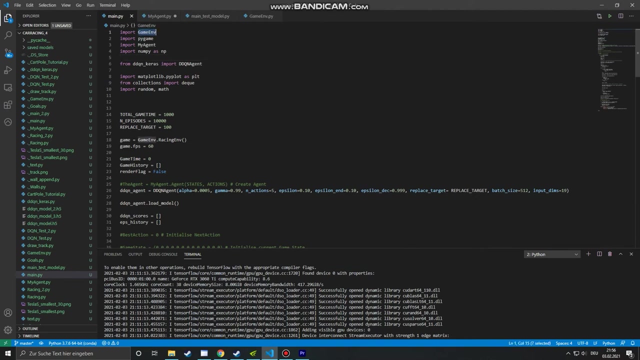 forward as well, and then we have a render function, which basically tells pygame how it should draw the certain frame of the game on the screen, and then, lastly, we have a close function. so this is the basic idea around the gaming environment. so, after setting up the gaming environment, the next thing that we need is the so-called agent. 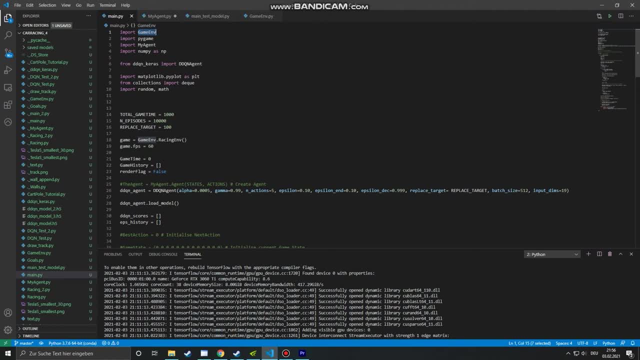 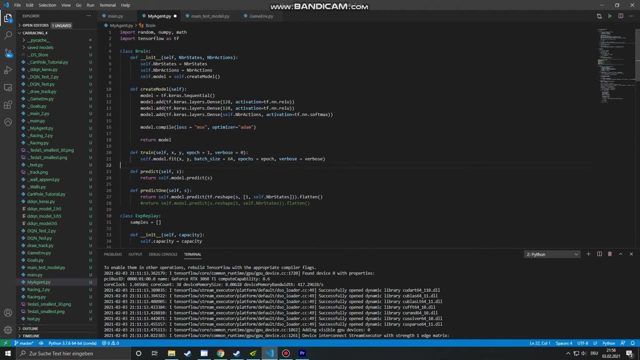 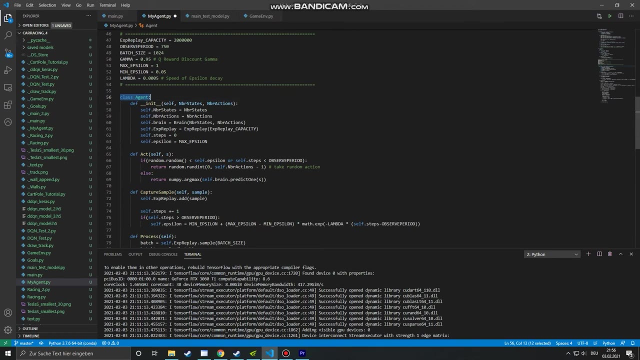 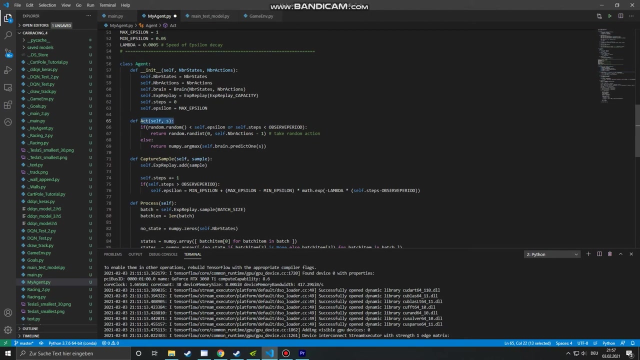 and this is basically the machine learning ai that controls the car. so let's have a look at it and it's written in this file here. so we have the class agent and it has different functions, like the act function, and it basically gets a certain observation data and then it acts either randomly or it predicts. 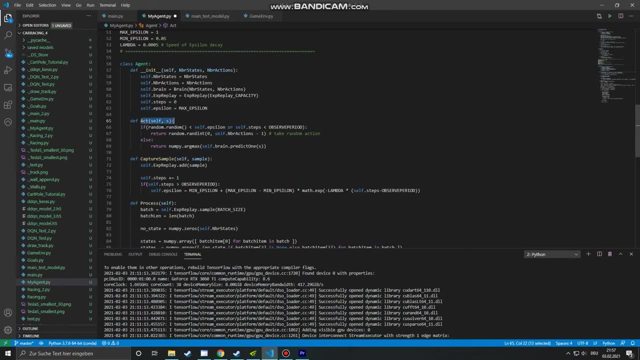 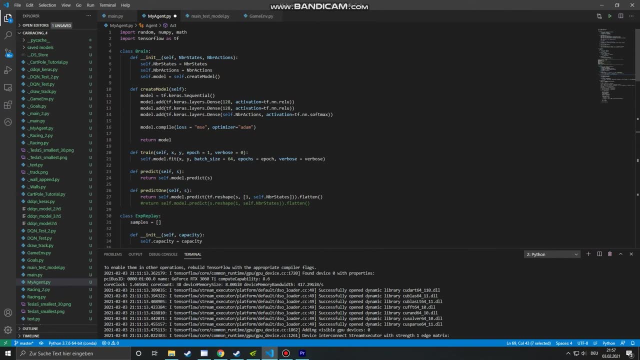 its action by using a neural network, and the neural network here is called brain. let's have a look at it and here we see the neural network that's behind the brain And, yeah, it has different functions to be trained and to predict its next action based on. 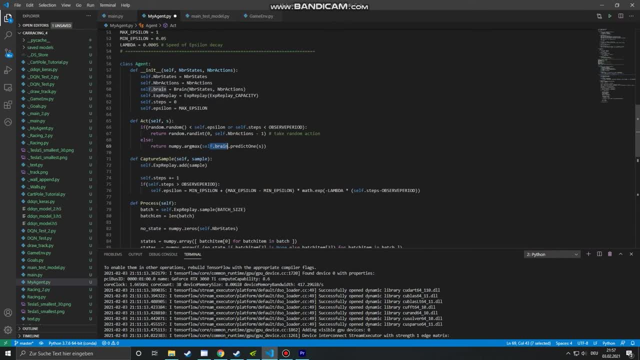 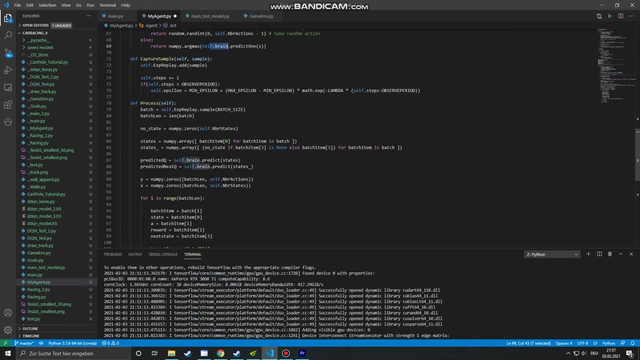 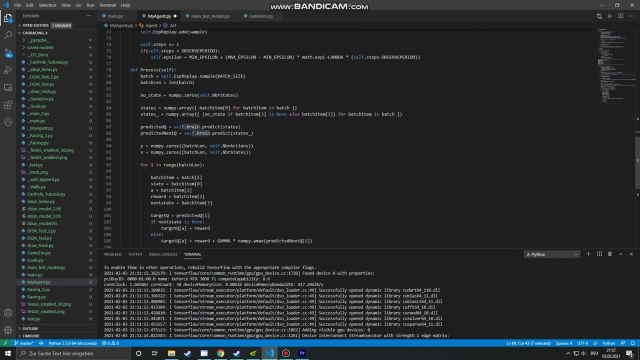 its observation And I don't want to go into a lot more details. If you're interested, please watch the video of cold bullets. He goes in a little more detail about how this algorithm works And after setting up the agent, let's see. 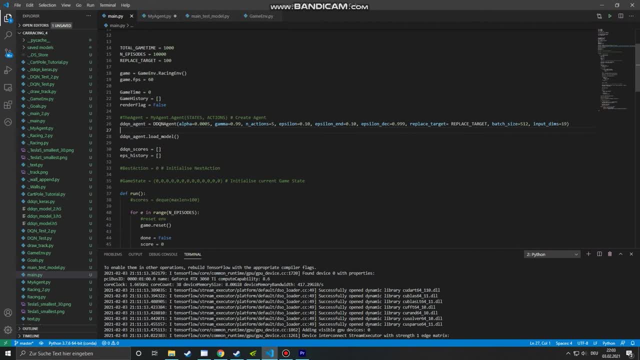 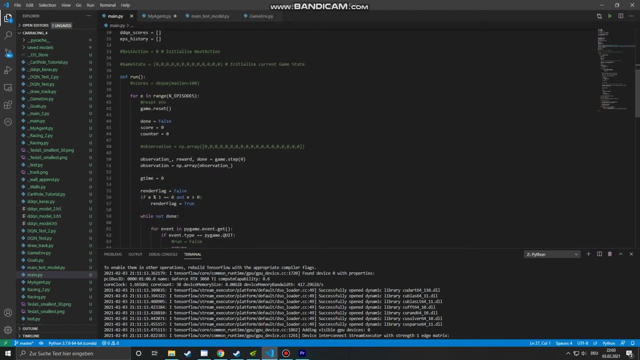 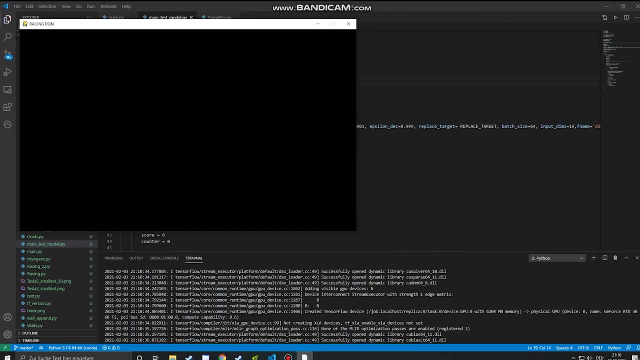 how the agent plays the game and trains inside the gaming environment. So the basic idea is learning. by doing so, the the agent gets to play in the gaming environment And through its observation, it gets better at playing the game Basically. So now let's have a look at what these observations. 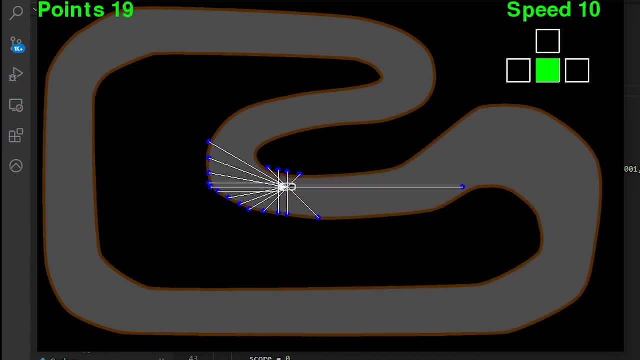 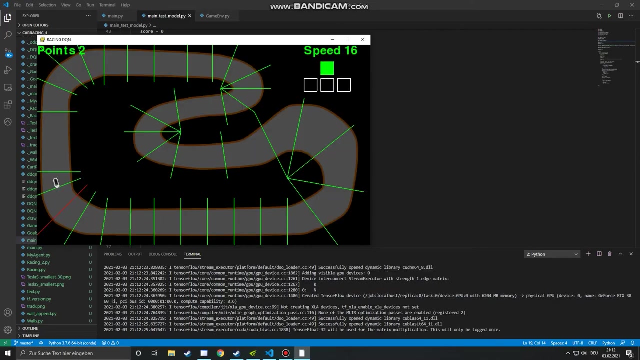 are. And now we can see what the the car is seeing basically. And it just measures the distance to the blue points And this is the only thing the car basically sees. The car also knows its own velocity. To measure the progress of the car, These green 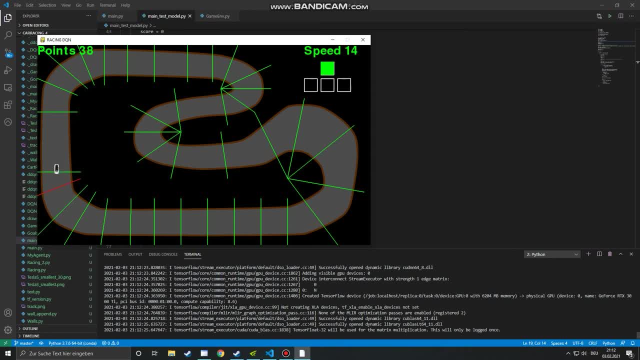 goals are used, And every time the car crosses the red line, the next goal gets activated, and so on and so forth. So that's it for this video. I hope you liked it and thanks for watching. And since I find it quite mesmerizing to watch the